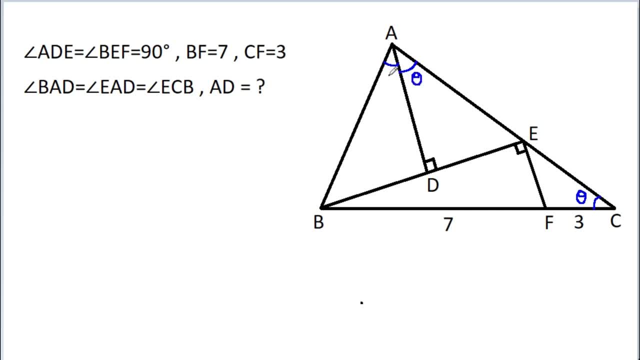 Suppose theta, Then we have to find AD. so suppose AD is X and inter angle ADE, it is ADE. this angle is 90 degree, this angle is theta. so this angle, it will be 90 degree minus theta. and 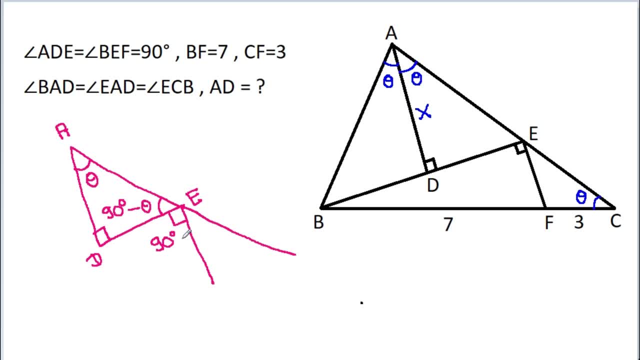 this angle it is 90 degree. so this angle it will be 180 degree minus 90 degree, minus theta minus 90 degree, and it is 180 degree minus 90 degree plus theta minus 90 degree. that will be theta. so this angle, it will be theta and. 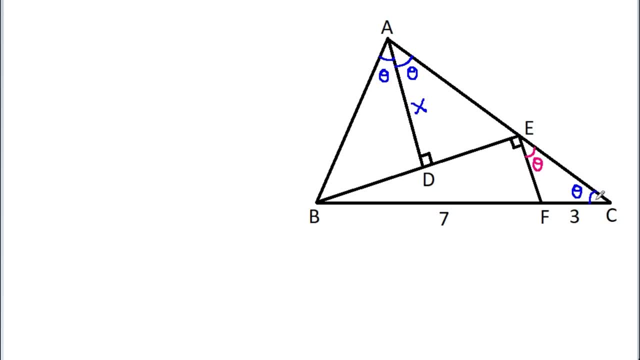 now inter angle: FEC it is FEC. These two angles, they are equal. So FC it will be equal to FE and FC it is 3. so Fe it will be also equal to 3. Fe it will be 3, and in any triangle, if this 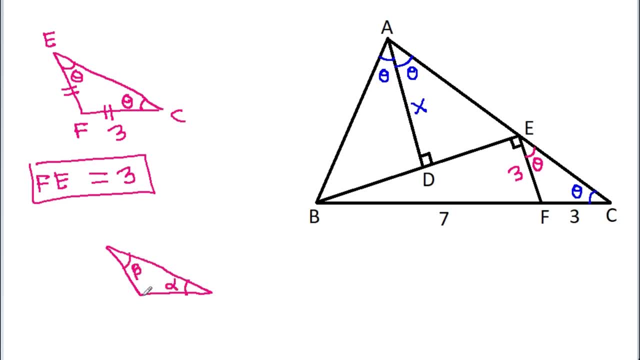 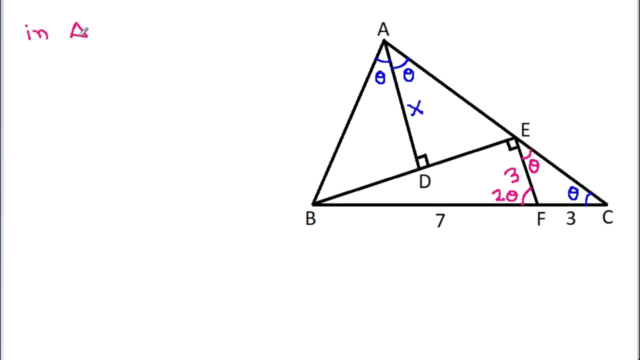 angle is alpha, this angle is beta, then this exterior angle, it will be alpha plus beta. so here, this angle, it will be theta plus theta, that will be 2 theta. and now inter angle: BEF it is BEF, this angle is 90 degree, EF is 3, BF is 7, so BE square plus EF square. 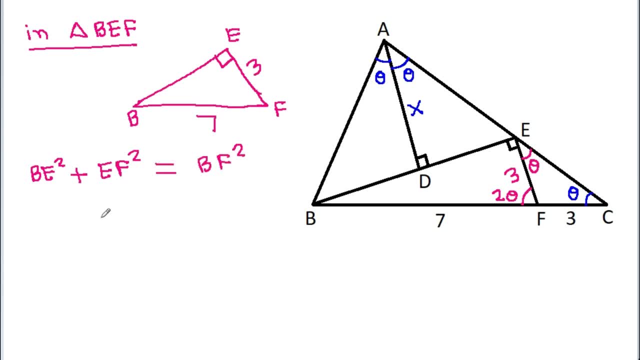 it will be equal to BF square by Pythagoras theorem. so BE square plus EF is 3 square, it is equal to BF is 7 square. and BE square plus 9 it is equal to 49. so BE square, it will be equal to 40. 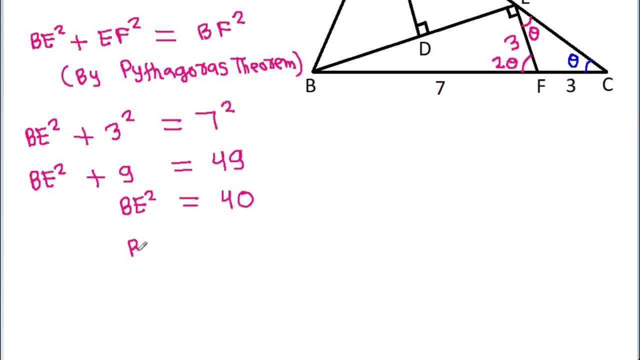 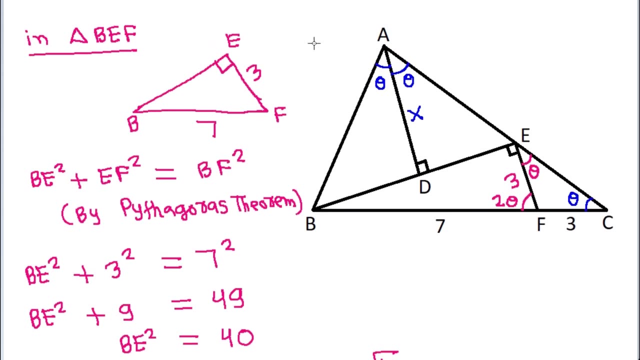 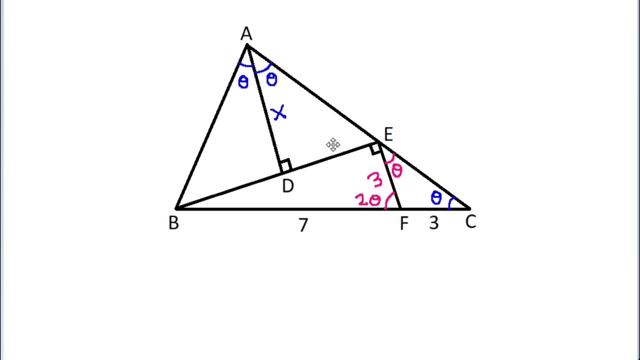 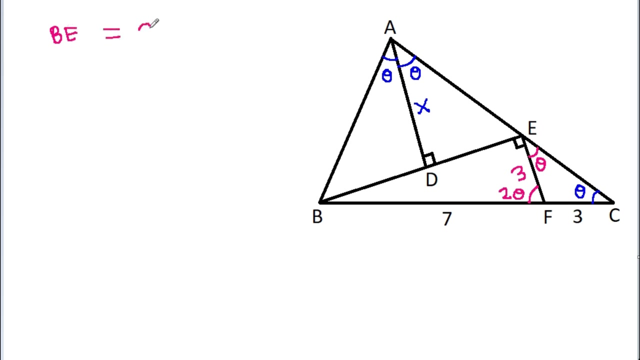 and BE, it will be equal to a square root of 40. that will be equal to 2 times a square root of 10. so we get: BEF is equal to 2 times a square root of 10. and now the triangle, ABD, it will be. 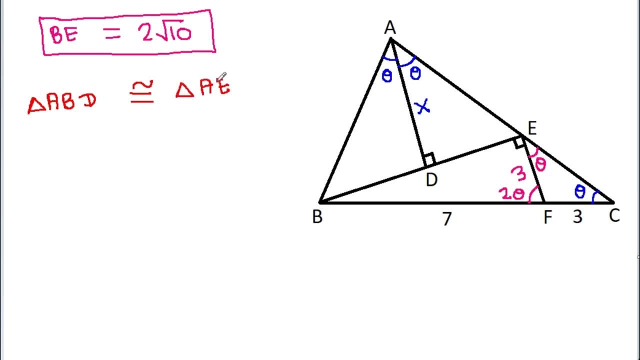 congruent to triangle AED, because angle BAD it is equal to angle EAD and AD is common, and angle BDA it is equal to angle EDA, so BD it will be equal to EAD and we have BE if 2 times a square root 10, so BD it will be equal to. 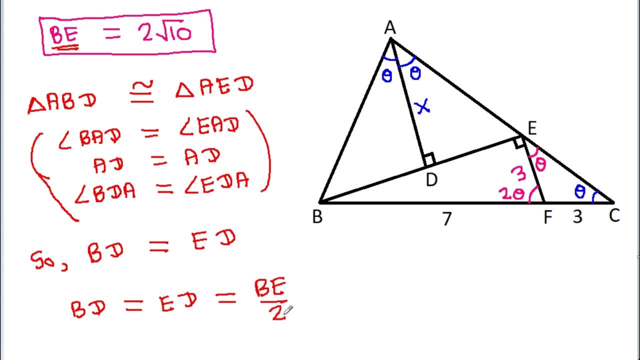 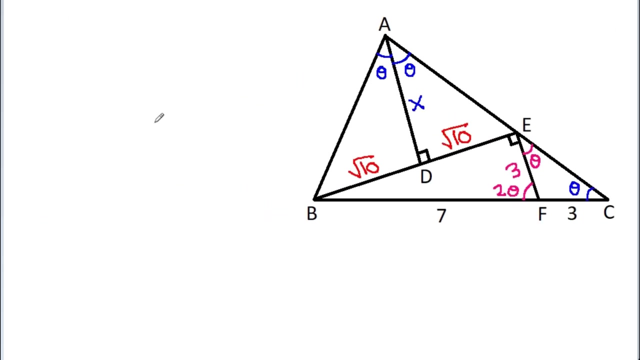 EAD, That will be BE by 2 and it will be 2 times a square root of 10. by 2 that will be a square root of 10.. so BD, it is a square root of 10.. and ed, it is a square root of 10. and now inter angle: abd. it is abd, this angle. 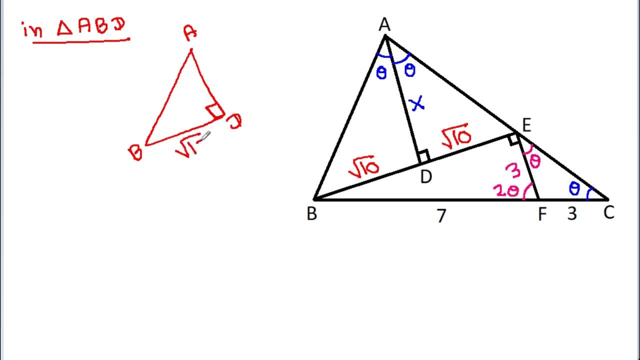 is 90 degree, bd is a square root of 10, ad is x and this angle is theta. so tan theta, it will be equal to bd by ad. that will be a square root of 10 by x. so x will be equal to a square root of 10 by tan theta. 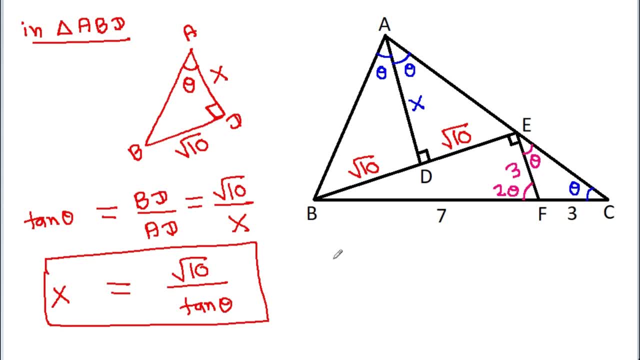 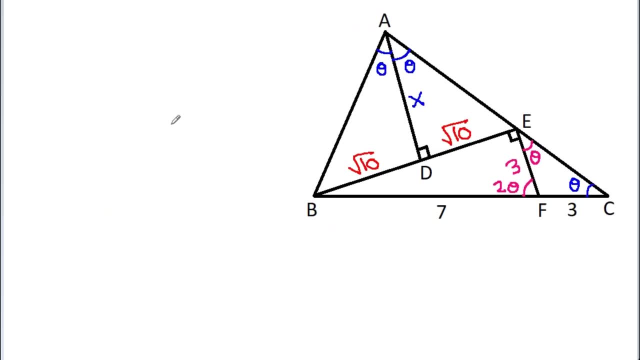